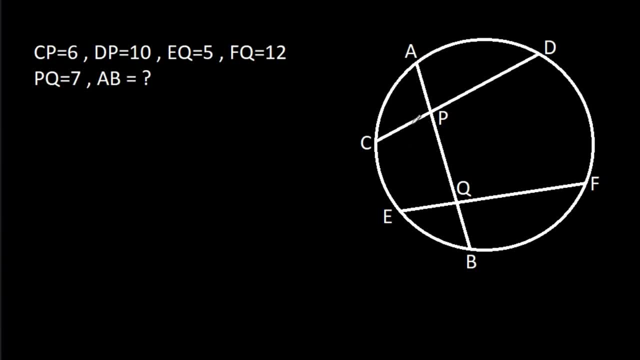 In this video we have been given that CP is 6,, DP is 10,, EQ is 5, and FQ is 12, and PQ is 7.. Then we have to find AB. So in any circle, if two chord, AB and CD, intersect at O, then AO times BO. 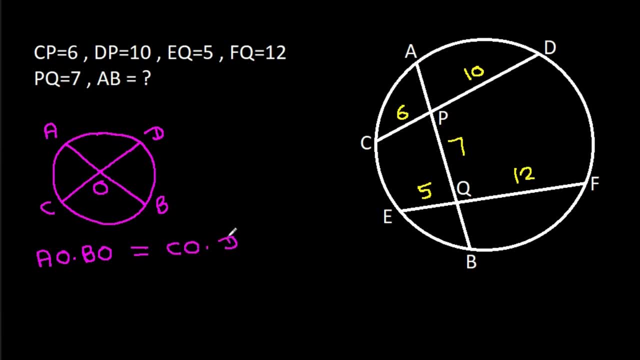 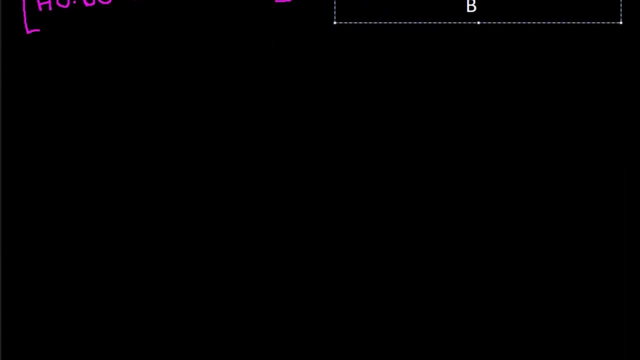 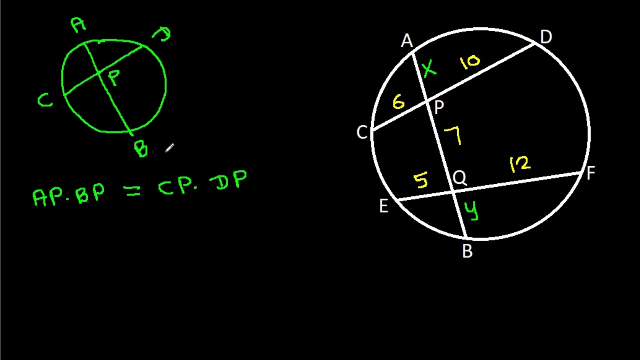 it will be equal to CO times DO. And here suppose AP is X and BQ is Y, then in the circle chord AB and Cen is intersecting at P. so AP x- BP it will be equal to, opposed to CP times, DP. 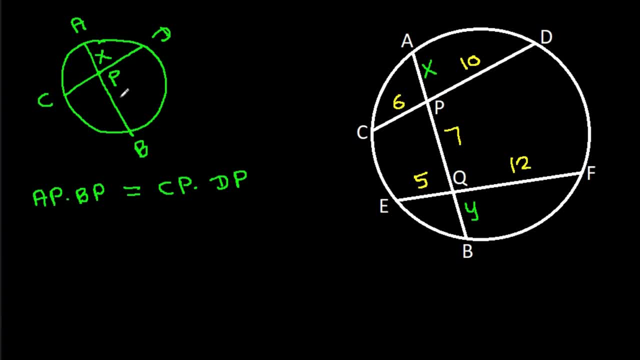 And AP is X, BP it is 7 plus Y, CP is 6,. conditions are showing: Should AB be equal to CD, Cp is 6 and Dp is 10.. So x times 7 plus y, it will be equal to 6 times 10.. And it is 7x plus xy is equal to 60.. 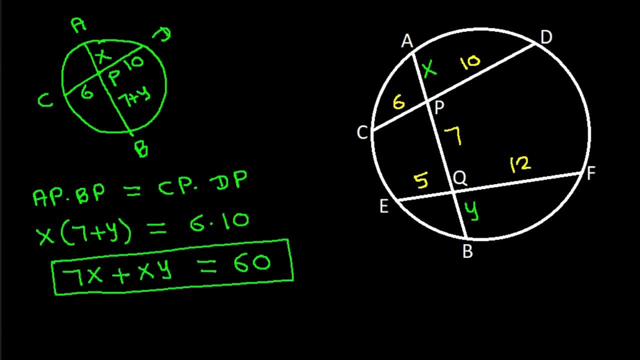 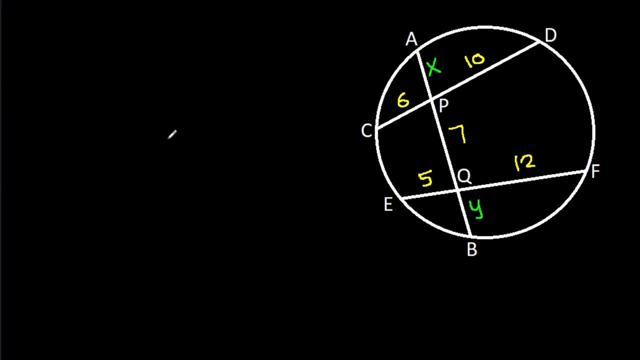 And also in the circle quad, AB and EF is intersecting at Q. So AQ times BQ, It will be equal to EQ times FQ, And AQ is 7 plus x, BQ is y, EQ is 5, and FQ is 12.. 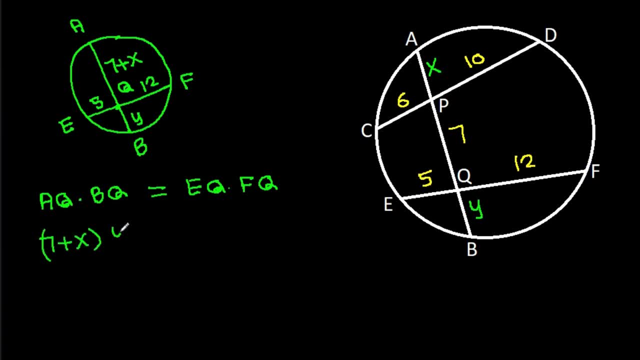 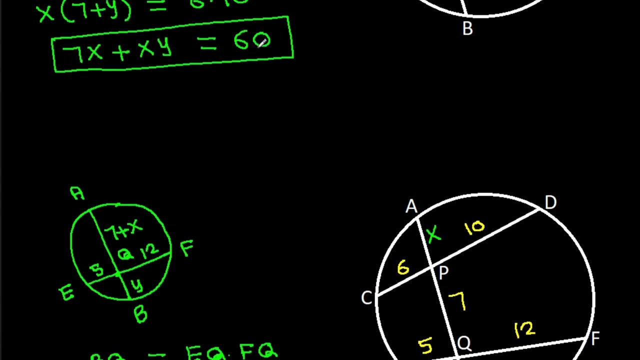 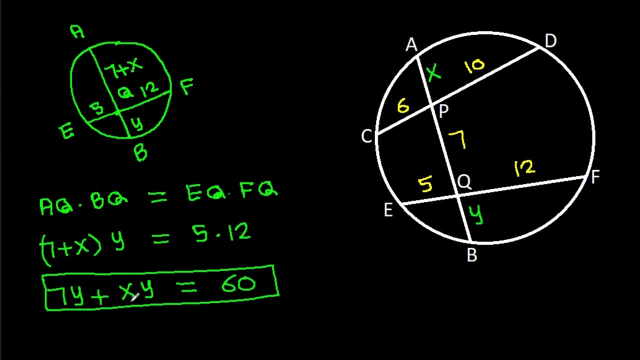 So it is 7 plus x times y is equal to 5 times 12.. And it is: 7y plus xy is 60.. And we have: 7x plus xy is 60.. Suppose it is equation 1.. And we have: 7y plus xy is 60. 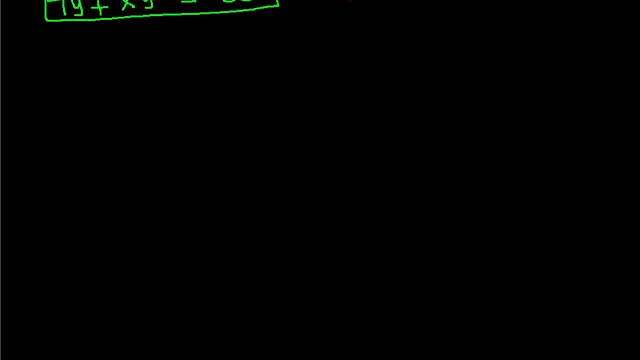 Suppose it is equation 2.. So from equation 1 and equation 2, we get: 7x plus xy is equal to 7y plus xy, that is 60. So 7x plus xy is equal to 7y plus xy and xy will get cancelled. 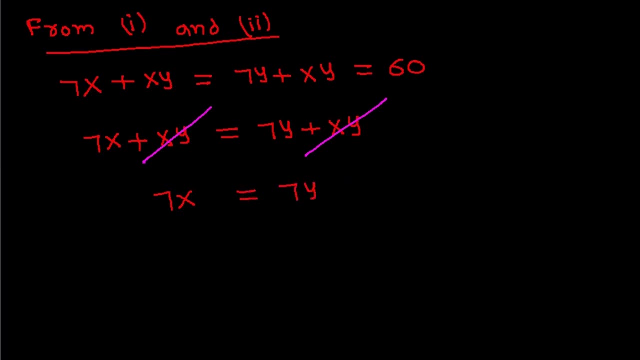 So 7x is equal to 7y and 7 will get cancelled, so x will be equal to y And we have 7x plus xy. It is 60. And it is 7x plus x times y is x. 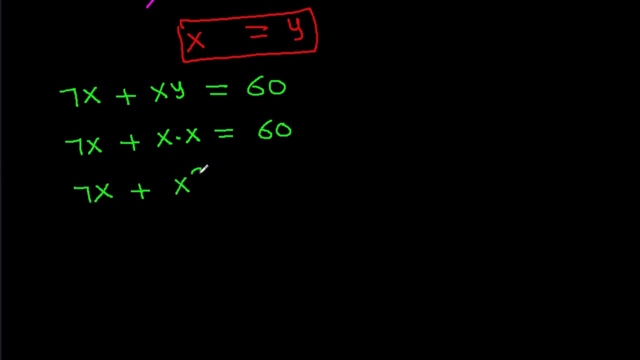 It is 60. And it is 7x plus x Ay is 60. And it is x Ay plus 7x minus 60 is equal to 0. And it is x Ay. Now it is x way and 7x it is plus 12x minus 5x minus 60, it is equal to 0, and here we can take. 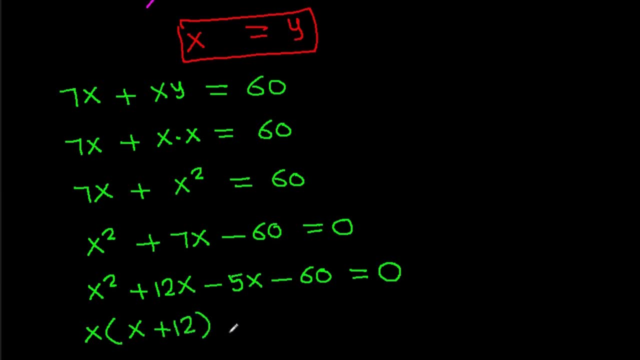 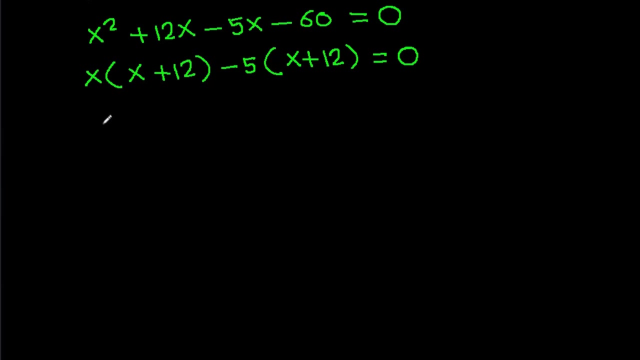 x common, and it is x plus 12, and here we can take minus 5 common, and it will be x plus 12,, that is equal to 0.. And now we can take x plus 12 common, and it will be x minus 5,, that is equal to 0.